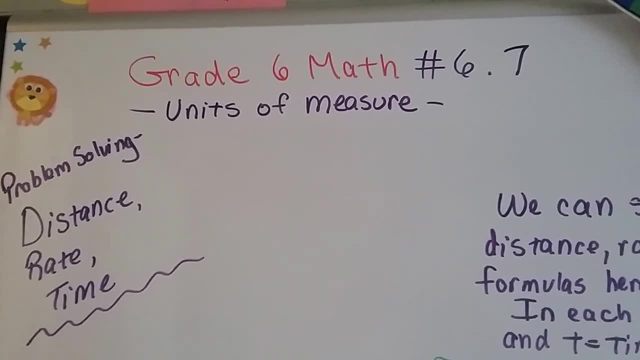 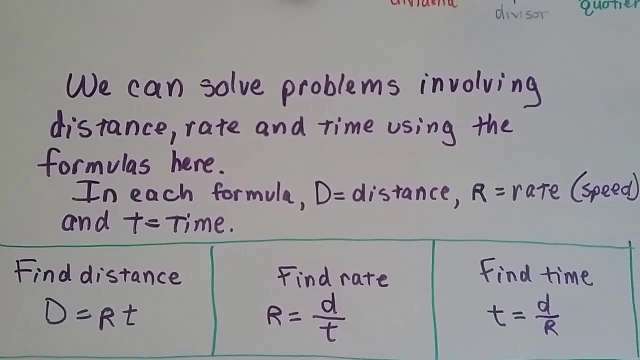 Grade 6 Math number 6.7, Problem Solving Distance, Rate and Time. We can solve problems involving distance, rate and time by using the formulas here. We can solve for distance, we can find the rate. 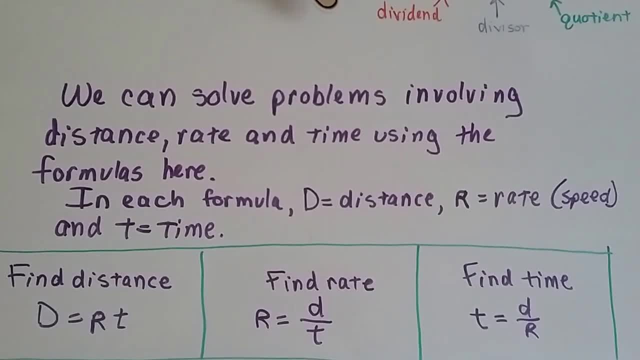 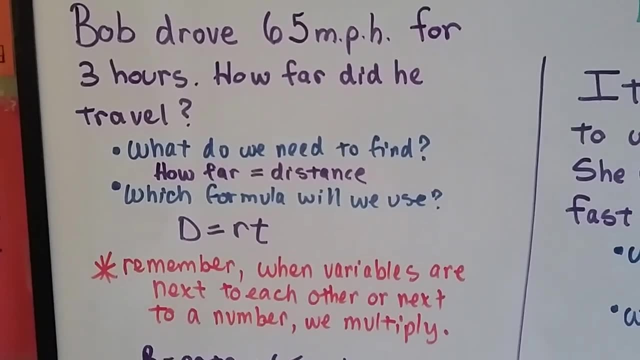 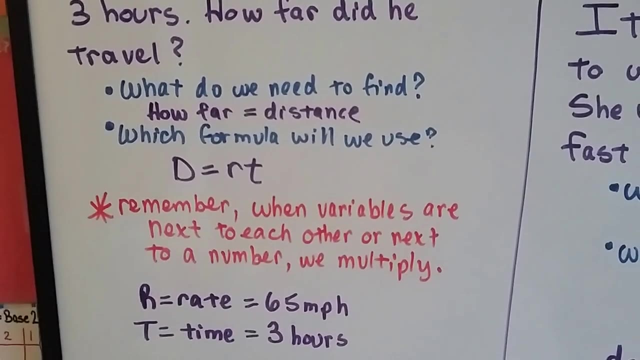 or we could find the time. D is distance, R is rate, which is speed, and T is time. Bob drove 65 miles per hour for three hours, so how far did he travel? Well, we ask ourselves, what do we need to find? It says how far, so that means distance. So that's the formula we'll use. 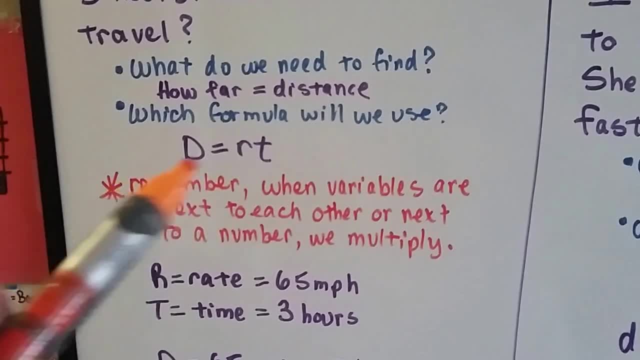 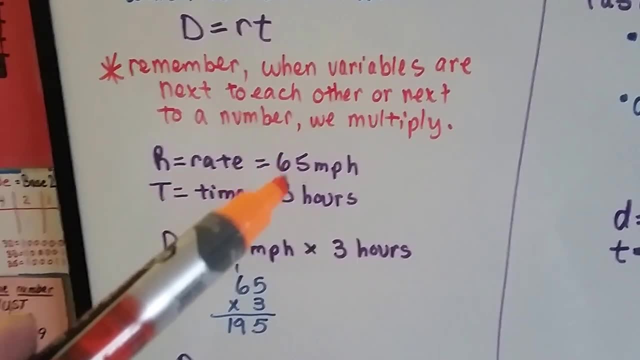 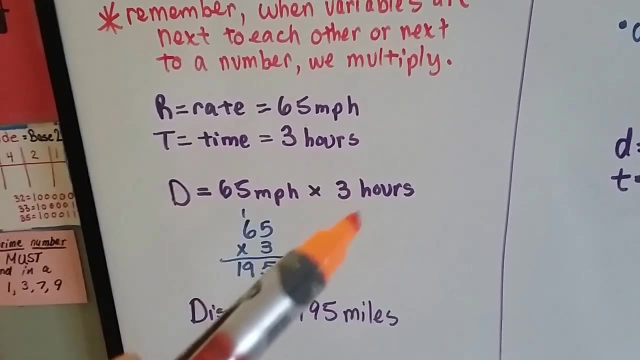 D equals RT. Remember, when variables are next to each other, that means we multiply. okay. R is the rate or the speed, and that's 65 miles an hour. T is the time, that's three hours. So we multiply them together: 65 miles an hour times three hours. 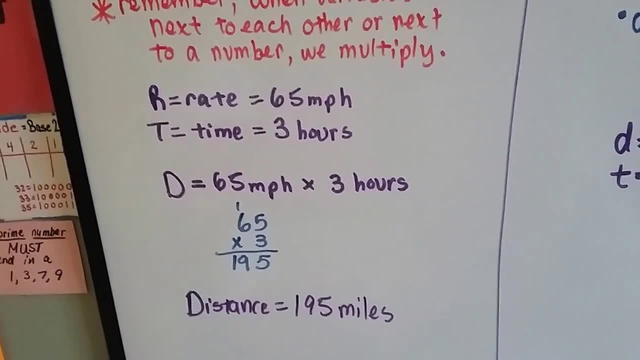 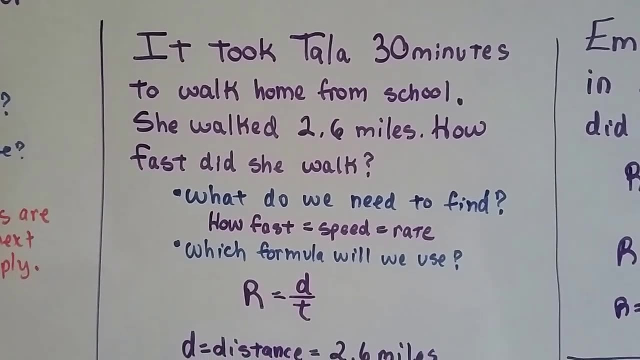 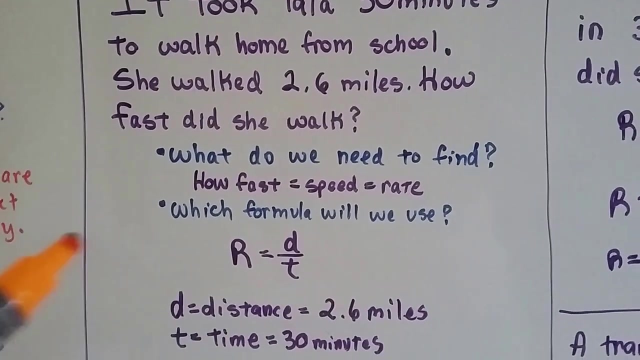 and we see it's 195 miles that he traveled. That's the distance. It took Tala 30 minutes to walk home from school. She walked 2.6 miles. How fast did she walk? Well, what do we need to find? We need to find her speed, how fast she walked. So which formula will? 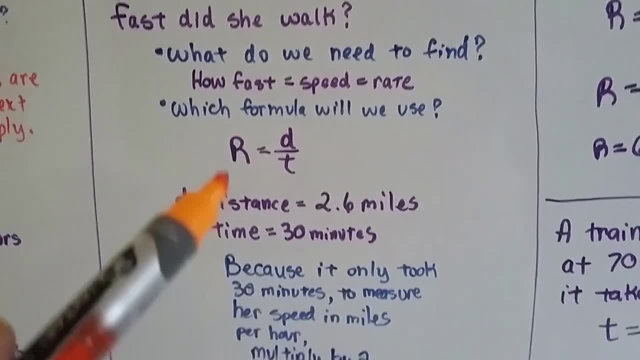 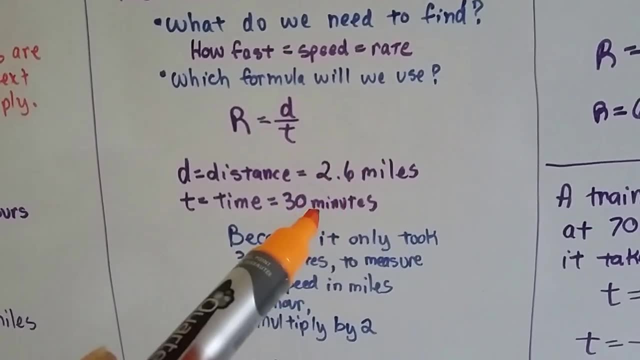 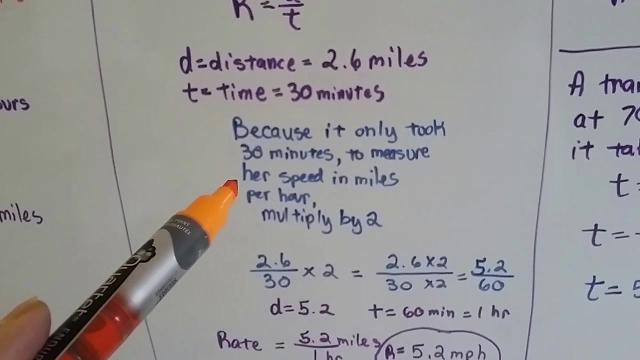 we use. We're going to use rate, because that's the speed. The rate is the distance over the time, the distance divided by time. so 2.6 miles divided by 30 minutes. Well, because it only took 30 minutes to measure her speed in miles per hour, we're gonna multiply it. 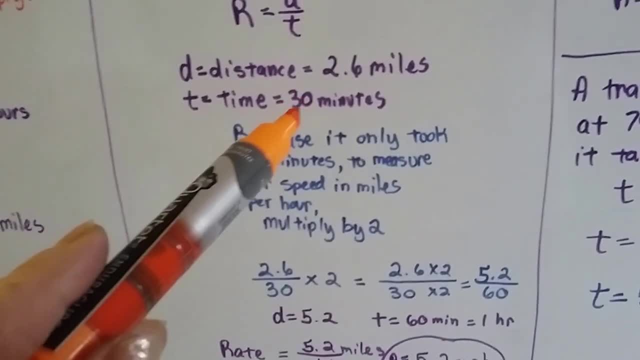 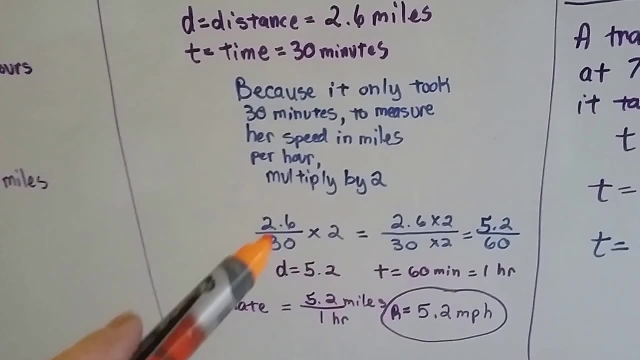 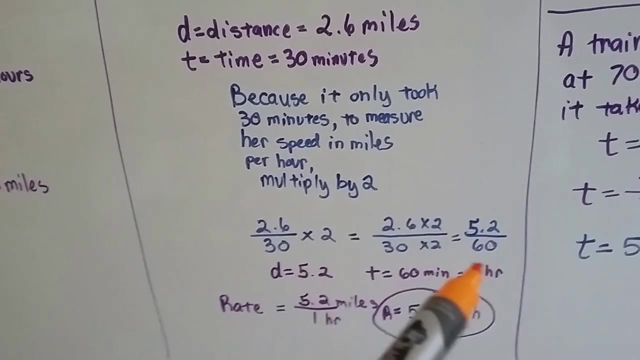 by 2, so it's 60 minutes. so it's a full hour. that way we'll be able to say how many miles per hour she walked. see, we multiply both by 2. 2.6 times 2 is 5.2, and 30 times 2 is 60 minutes. so now we know she did 5.2 miles in 60 minutes, which is 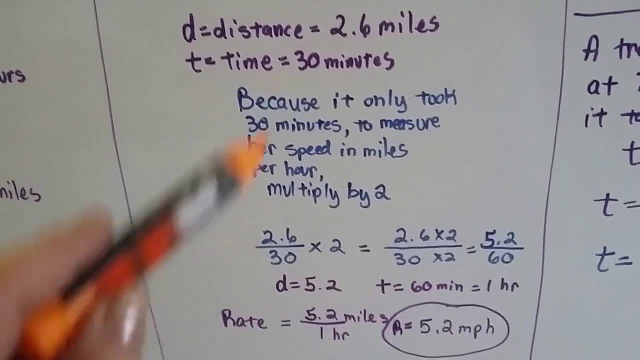 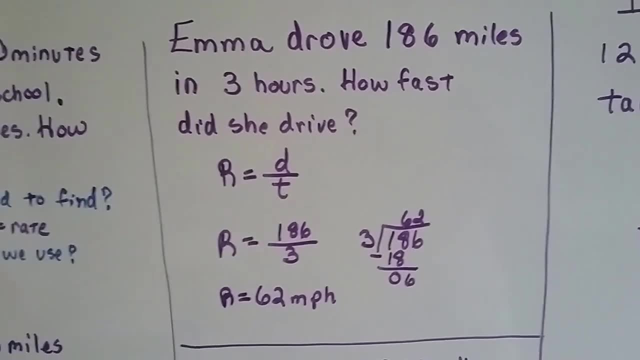 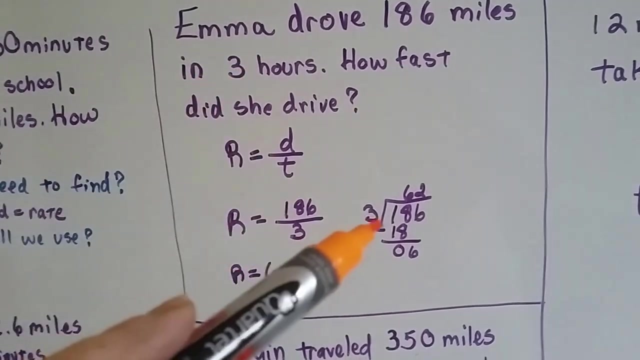 one hour she walked 5.2 miles an hour. that was a little different, wasn't it? Emma drove her car 186 miles in 3 hours, so how fast did she drive? same formula: we put the 186 miles over the 3 hours and we divide 186, divided by 3 is 62. we.